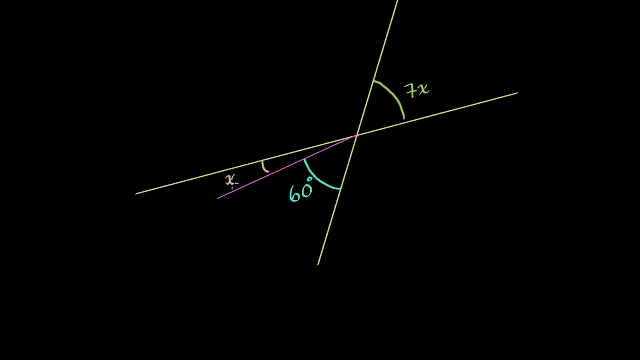 and the measure of this angle right over here is x. So let's try to figure out what all of these angles are. So to do that, we have to figure out what x is, And there's a big clue here, because the 60 degree angle plus the x angle, 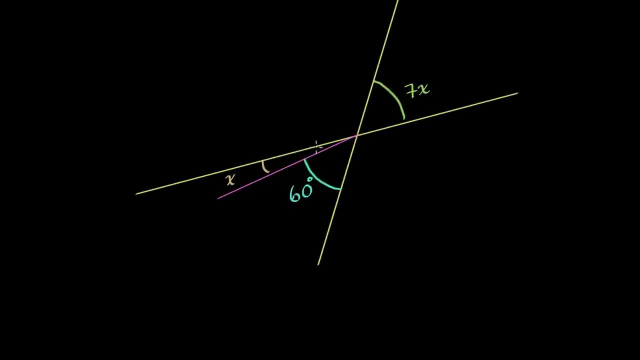 they're adjacent And if you add these two angles together their outer rays are vertical angle with this seven x angle. So we could say- and just to visualize it a little better, let me color it in- So you see that this actually let me do it this way. 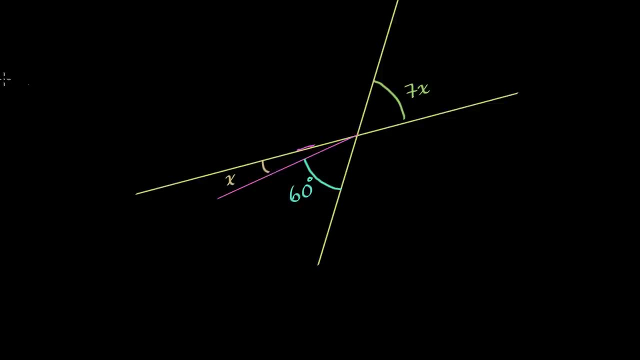 You see, you see that this angle out here- let me do it in a color I haven't used yet- this entire angle right over here, which is going to be 60 degrees plus x, that's a vertical angle. with this angle, 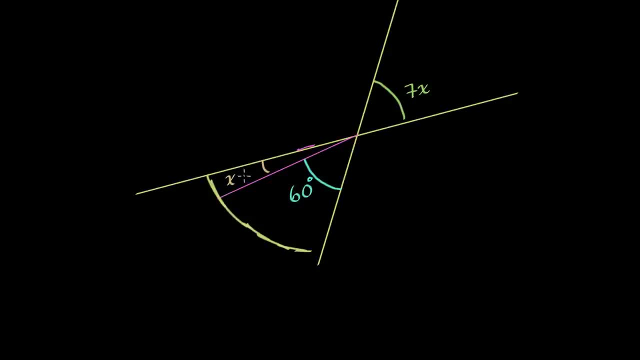 the one that has measure seven x. So we could say that 60 degrees plus x is equal to seven x, because vertical angles are equal. So let's write that down, We get 60, and we'll assume that everything is in degrees. 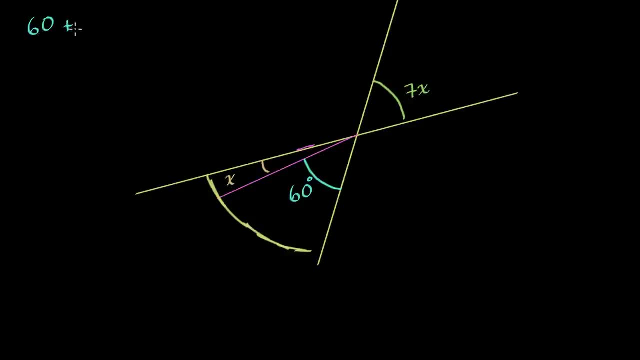 60 plus. let me do that in this other color. 60 plus x is going to be equal to seven x, And now we just have to solve for x. So the simplest thing to do would be to get all of our x's on one side of the equation. 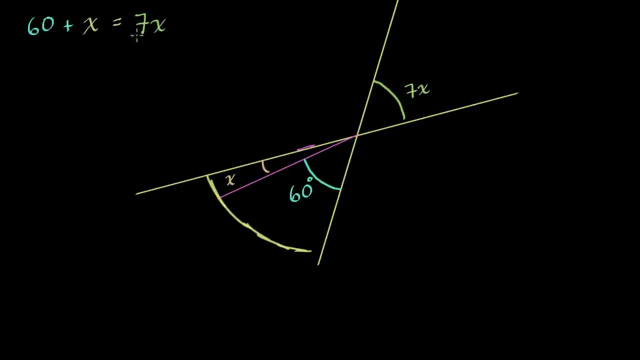 I've already gotten seven x's on this side, this right-hand side, so let's get rid of all of the x's on the left-hand side. And the easiest way to get rid of this x is to subtract x from the left-hand side. 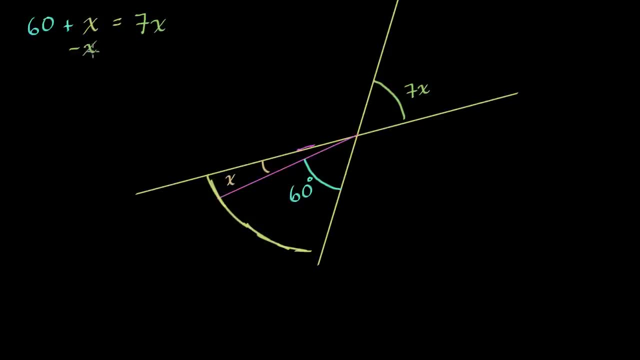 But of course, in order to keep it an equation, we can't just do something to one side, otherwise it won't be equal anymore. We have to do it to both sides. So let's subtract x from both sides, And on the left-hand side we are left with just the 60.. 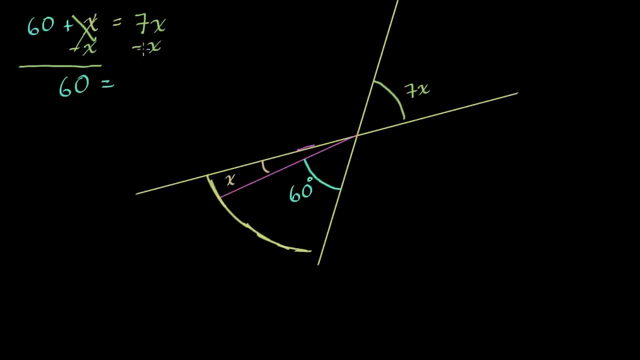 So we're left with just a 60, and then that is going to be equal to seven x minus x. So I have seven of something, and when I get rid of one of them I'm going to have six of that something left. 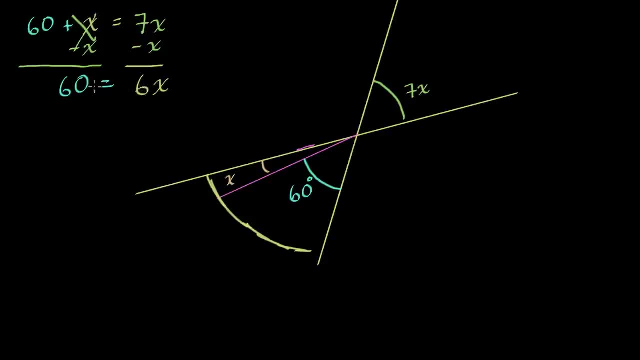 So that's going to be equal to six x. So we have six times something is equal to 60.. You could probably figure that out in your head, but I will do it a little systematically. We can divide both sides by six to solve for x. 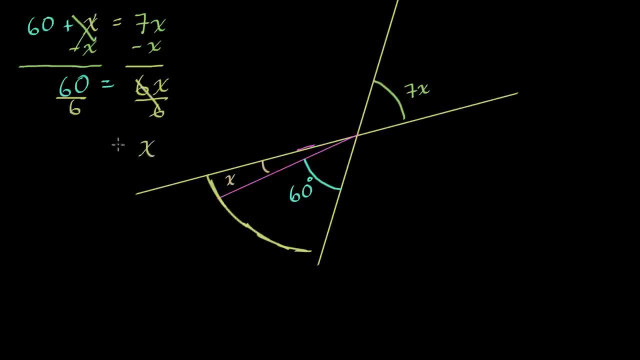 So let's do that and we would be left with: x is equal to 60, divided by six is 10.. And we reminded ourselves that everything was in degrees, And we could even do that here. This was in degrees, this was in degrees. 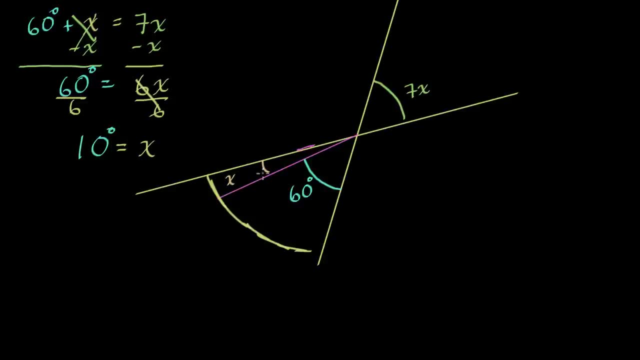 and so this is in degrees right over here. So the measure of this angle right over here is 10 degrees. So this one right over there is 10 degrees. This is, of course, 60 degrees. You add them together: 60 degrees plus 10 degrees. 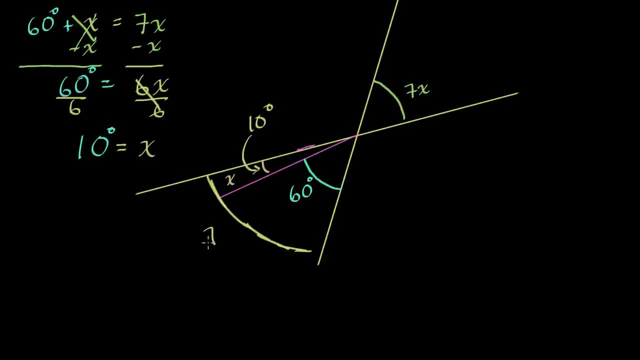 is 70 degrees. So this bigger angle right over here is 70 degrees And of course, this one over here it's a vertical angle. it's going to have to be the same and we see that Seven times x, seven times 10 degrees is 70 degrees as well. All right. 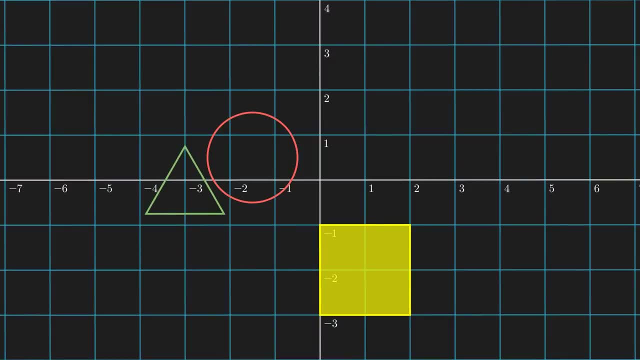 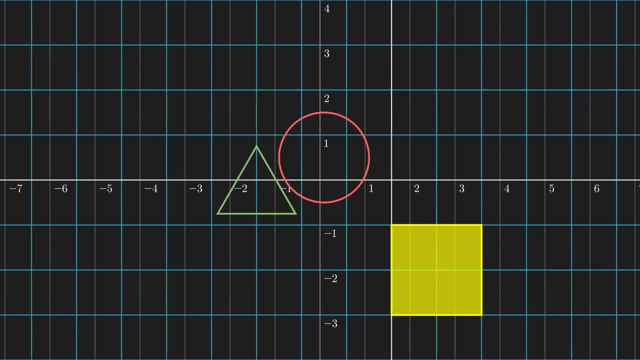 While I was working on another video, the topic of special Euclidean group came up, which, roughly speaking, is a collection of all translation and rotation in space, And translations and rotations do not commute with each other. If we translate two steps to the right, then rotate 90 degrees about the origin. 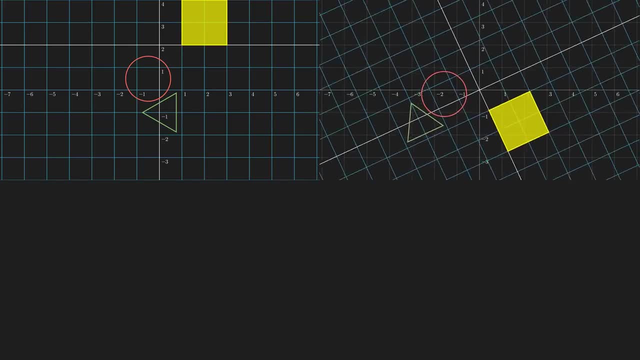 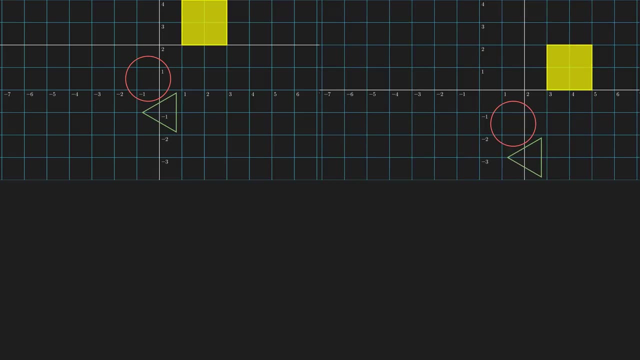 then we would get a different result. if we do them in reverse, which is to rotate first, then translate two steps to the right. Now the real interesting thing is: either way we compose these transformations, they end up being rotations about some other point in space. 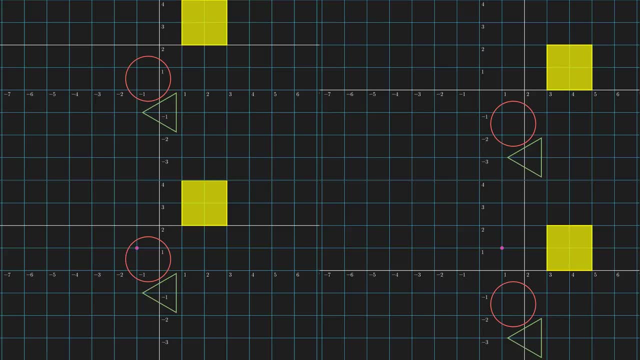 And that raises couple of questions. Why did they end up being rotations about some other point which is negative, 1 and 1, and 1, 1 respectively? And the more important question is: can we come up with a formula for rotating about any point?